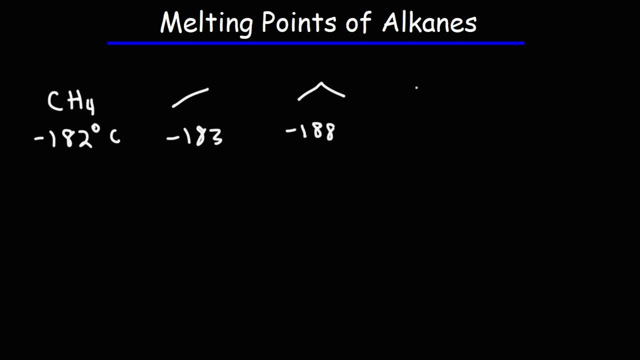 that's negative 188.. Next is butane coming at negative 138.. And then we have pentane, which is at negative 130.. Followed by hexane. The melting point for hexane is negative 95. And then for heptane, negative 91. 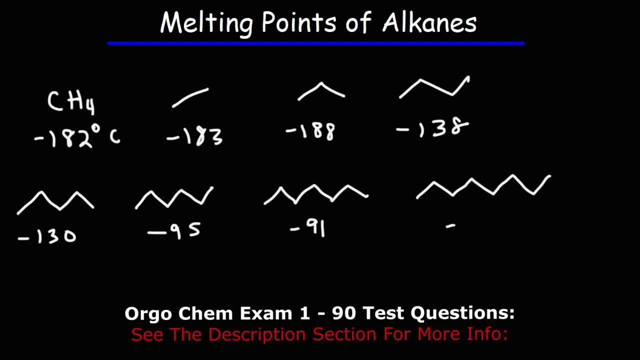 And for octane it's negative 57.. Now for nonane, which has 97.. For fine carbons, the melting point is negative 51. And for decane, negative 30. Now notice the general trend for the melting points of our cane. 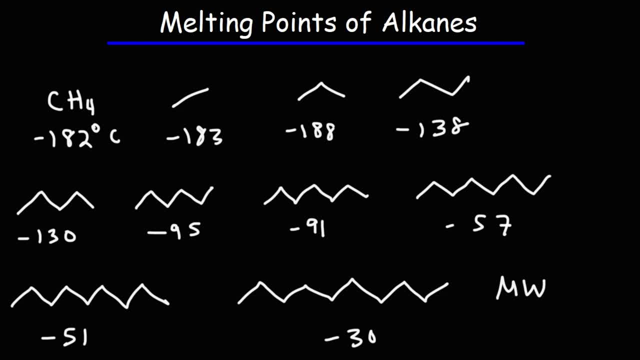 As the molecular weight increases, as we add more and more carbon atoms to the chain, the melting point, generally speaking, will increase. So the trend is very similar with boiling. We know that for longer hydrocarbons the boiling point increases. 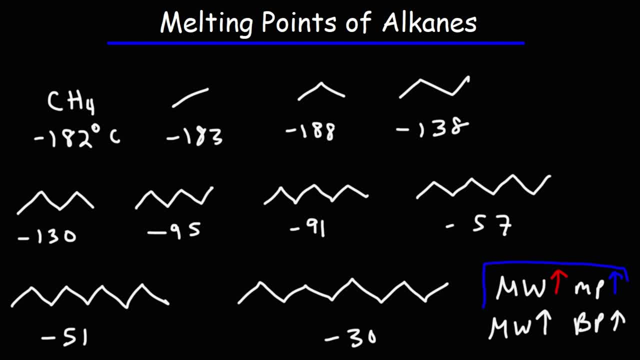 But the melting point of alkanes has some unusual features. First, the trend doesn't really work for the first three alkanes: methane, ethane, propane. As we go from negative 182 to negative 183, the melting point is actually decreasing. 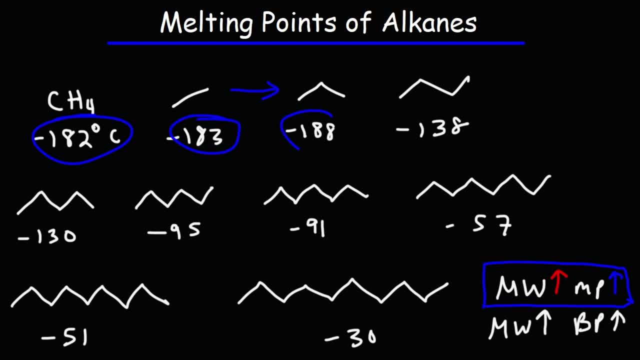 And going from ethane to propane it decreases even more. So propane has the lowest of the melting points of the alkanes listed here, which is kind of strange. But after propane the trend follows the molecular weight. As you add more and more carbon atoms, the melting point will increase. 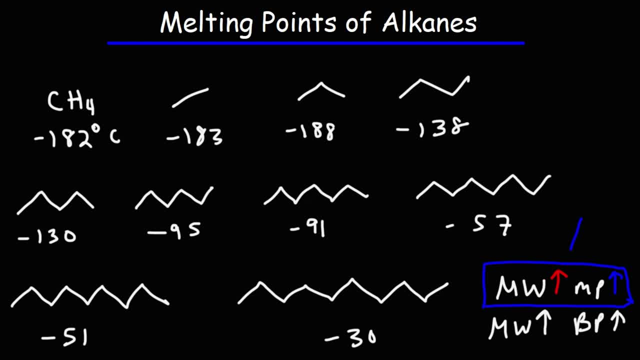 Now there's something else that we need to pay special attention to, and that is the drops in the melting point between certain alkanes. notice that as we go from propane to butane, there is a huge drop in the melting point. i mean not a huge drop, but rather a huge increase in the melting point.